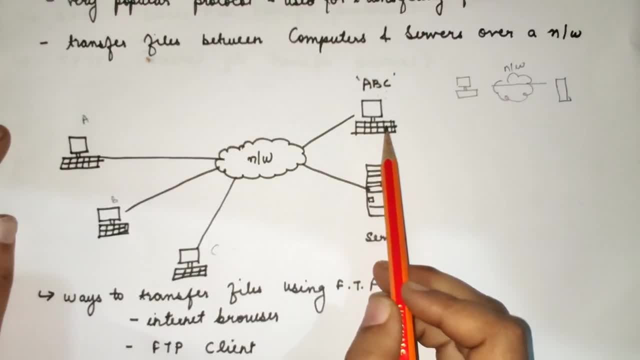 So if this ABC wants to send, wants to upload A file which have to make available for everyone for downloading purpose, Then what ABC will do? ABC will upload the data or that particular file to this server through the network. in a similar way, This holds A, B and C can access the data using this FTP server through the network. 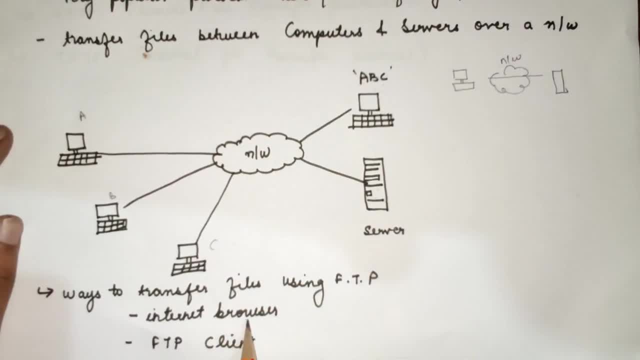 There are two ways, for there are two ways to transfer file using an FTP. First is an internet browser and the second one is an FTP client. We will see what is internet browser And how FTP client is used for transferring the data. See how this internet browser work. 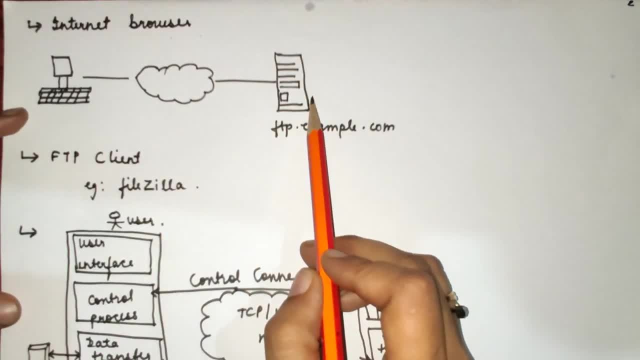 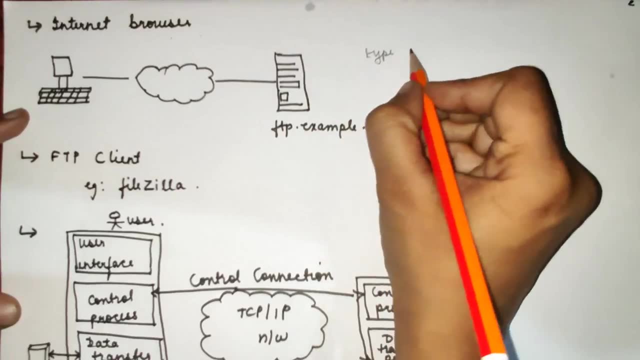 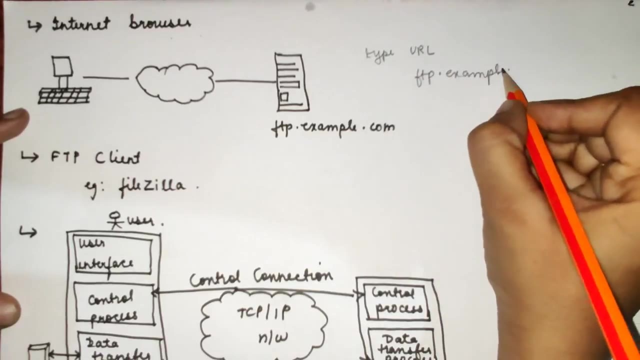 For example, someone has uploaded a songs, MP3 files, on this FTP FTP server and we want to download it. What we are going to do? We are going to type in your URL. You have to just type FTP dot, for example, some site, but it is going to be FTP. 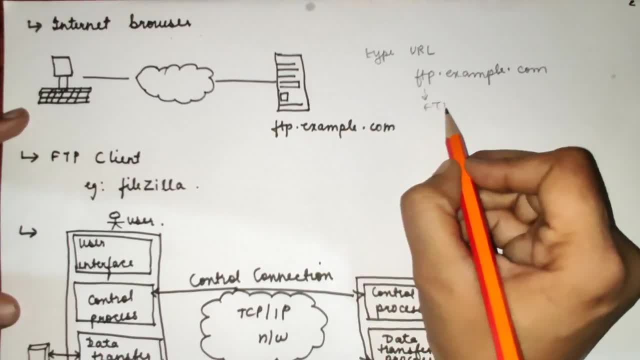 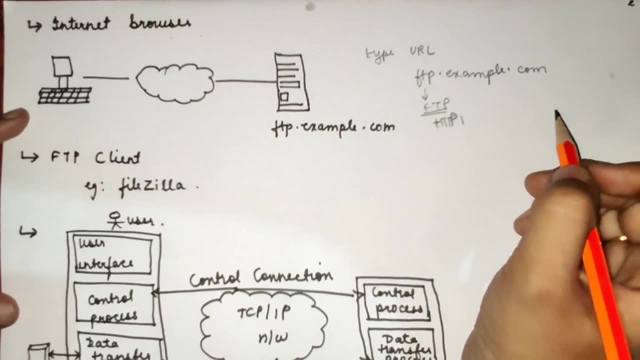 The extension, as you can see, is an FTP. It is not HTTP. Normally what we type we type HTTP, but here you can see it is an FTP. So in this way you have to write down the prefix FTP and that particular site, your name, in the URL. 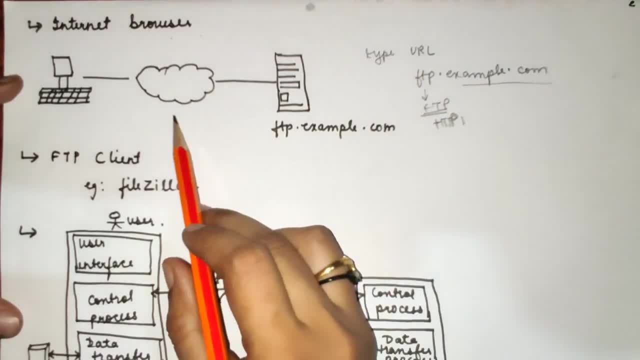 Okay, then you can easily download it. It is like a browsing for the in the particular file, like we normally Google it. Similarly, you can use using the internet browser, but the extension is going to be FTP. Now what is this FTP client? 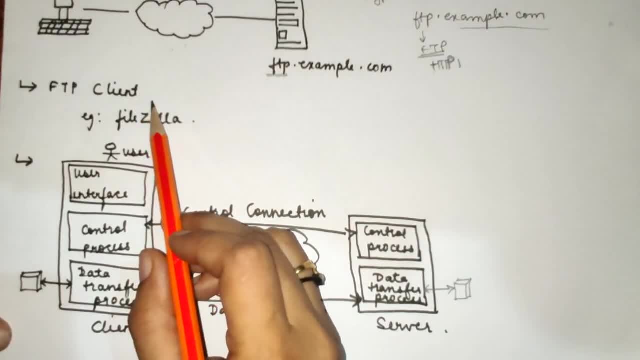 There are various FTP clients available. A very popular free FTP client you might be heard about is an FileZilla. FTP client provides a graphical user interface and a better way, or you can say a better overall experience, than an internet browser. So in this figure, in this figure you can see there is one client and a server. 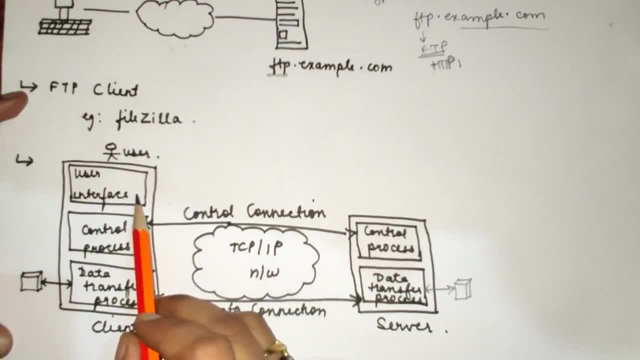 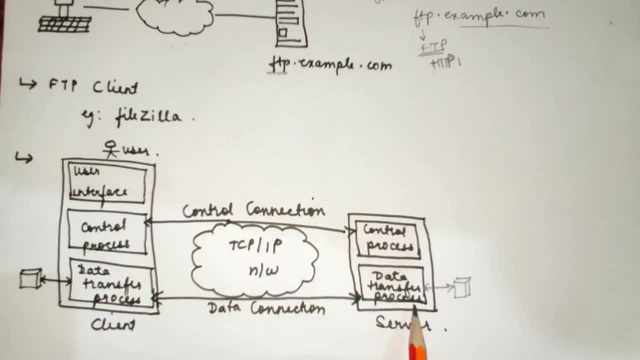 There are three components. There are going to be three component at a user side: user interface, control interface Or you can say control process and a data transfer process, Whereas in the server there are only two. One is control process and the second one is the data transfer process. 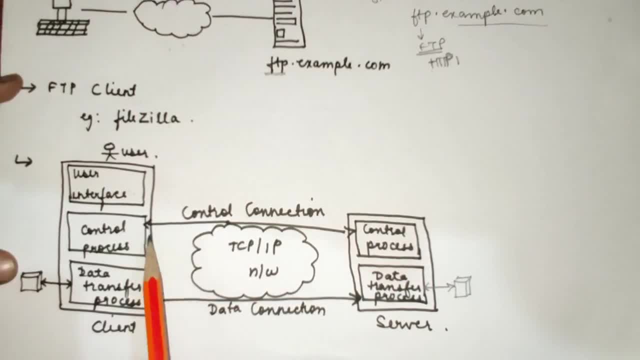 FTP usually differ from other client server application. FTP establishes two connection. One connection is used for controlling and one connection is used for data connection. So you can see, one is the control connection and the second one is a data connection. Control connection: Control connection has been developed between the control processes of client and a server. 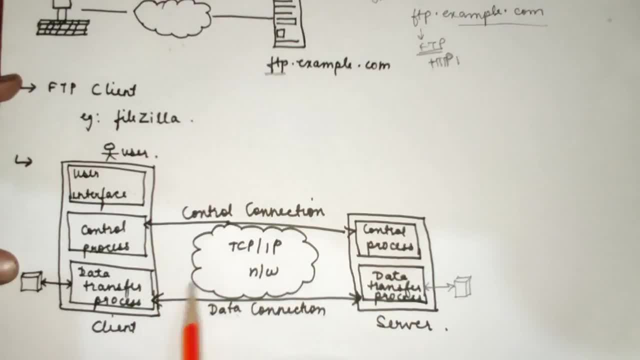 Whereas data connection is going to be builded between the data transfer processes of client and a server, Control connection remains connected during the entire connection. Through the control connection, we can transfer a line of commands and a line of responses at the same time, And this is going to use a port number 21.. 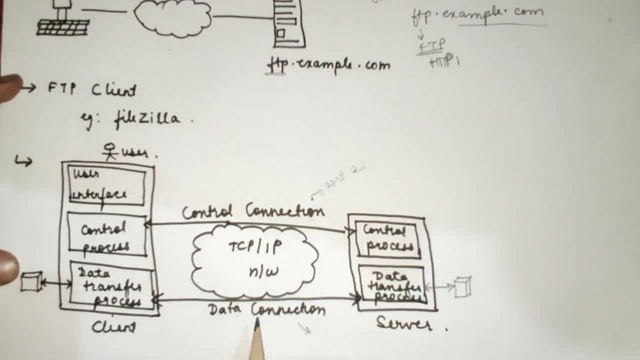 Whereas what happen in a data connection? Data connection is going to open and close for each file transfer. Whenever we want to transfer the file, the data connection is going to be open And once we transfer the data, the connection is going to be break. 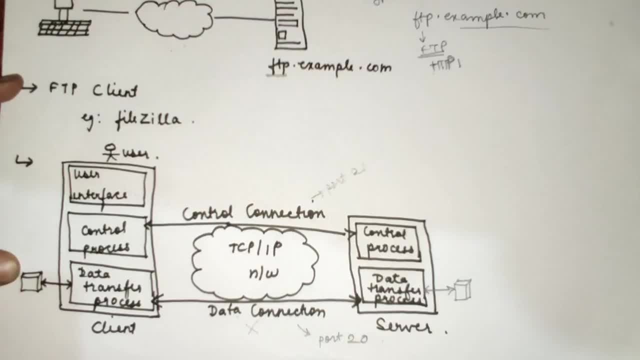 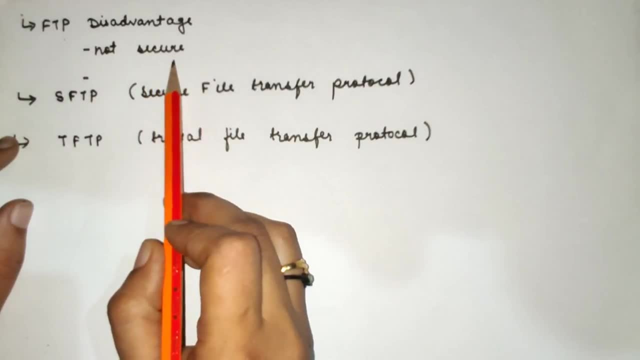 And it is going to use the port number 20.. But this FTP has some disadvantage. It is not a secure protocol, Means if we want to transfer the data in an encrypted form, it is not allowed. The data is sended in a clear text. 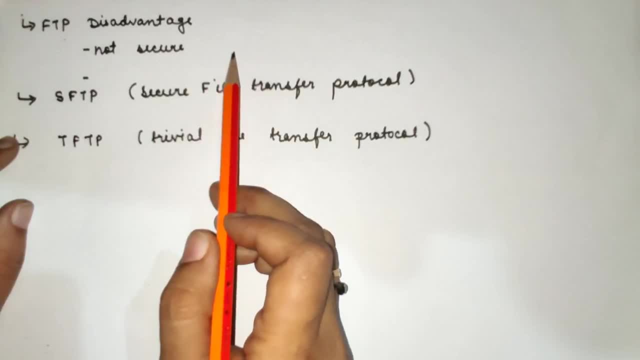 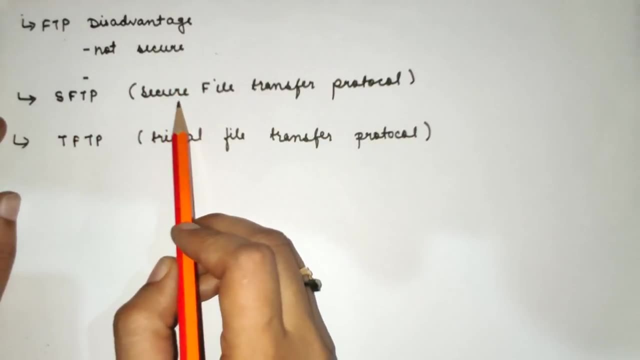 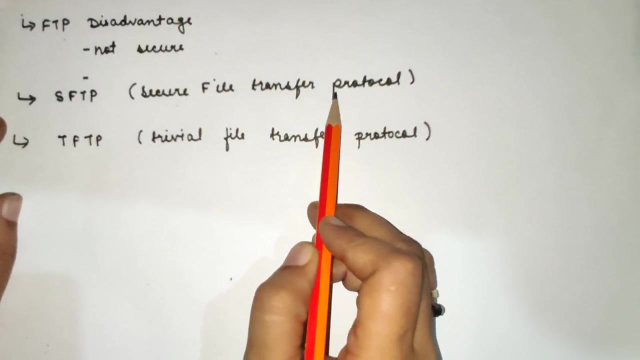 Hence it should only be used for a limited purpose. So, because of this advantage, another file transfer protocol- or you can say that as FTP- secure file transfer protocol- came into the existence. What happen in this? It is same like an FTP, But it adds a layer of security to it. 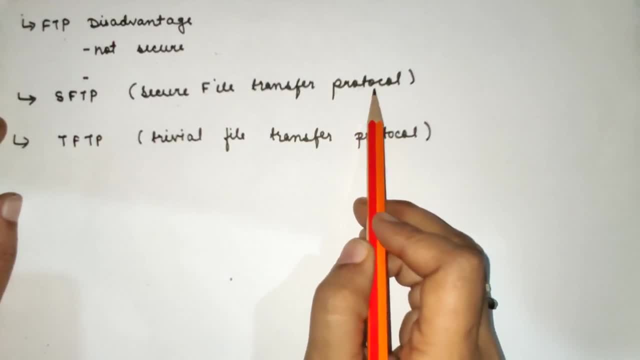 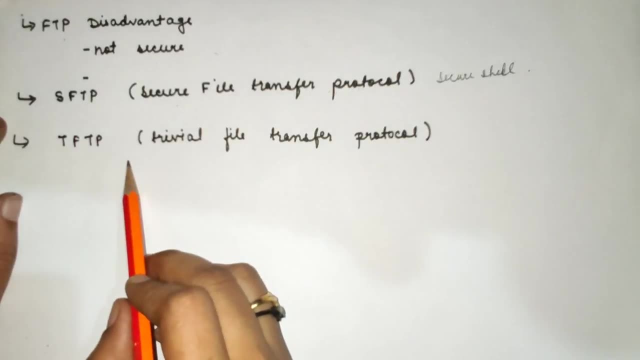 Means the data is going to be encrypted in secure FTP using a secure shell. One more FTP- that is trivial file transfer protocol- is there. What is this trivial file transfer protocol? It is used for transferring the file within the local area network. Means like FTP, it is used to transfer the files over the internet. 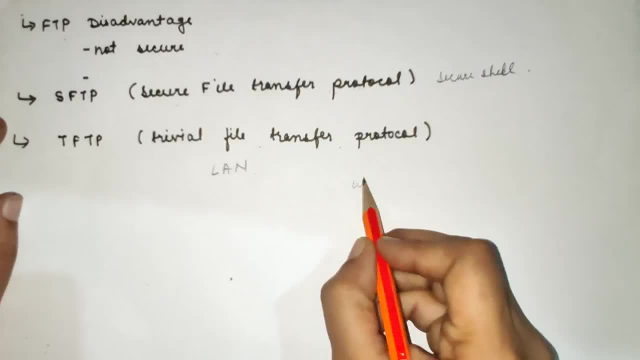 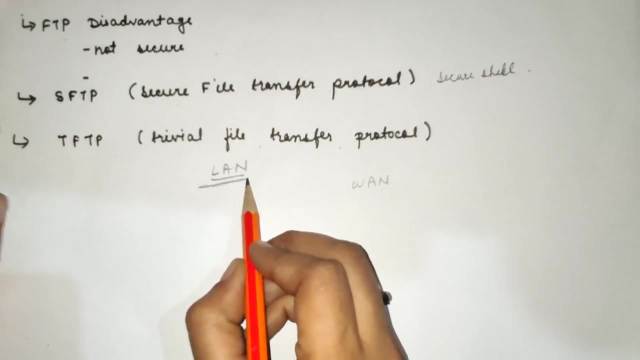 Means we are transferring the data all over the internet. Means we are using wide area network. But this is only used for the local area network. If we want to transfer the file within the local area, at that time also we can use this trivial file transfer protocol.